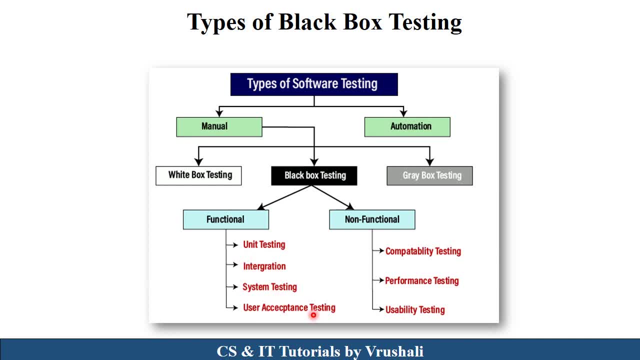 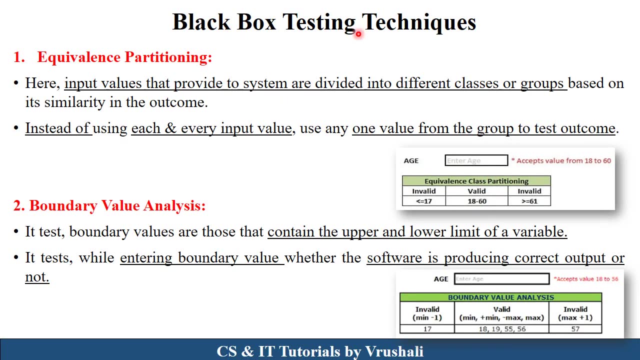 into the unit integration system and acceptance testing, Non-functional testing divided into the compatibility, performance and usability testing. We will discuss these types of testing with example in next sessions. The next topic is black box testing techniques And the first technique is equivalence partitioning. Now see here in this example, Suppose in: 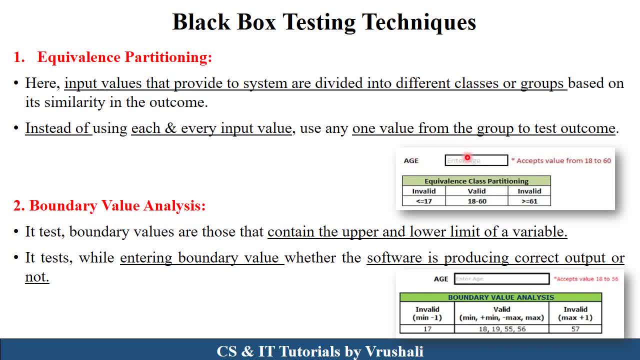 any registration form there is a option age and particular text box is there. Now this text box accept a value from 18 to 60, age only Right. So at that time, for testing purpose, tester use equivalence partitioning technique. They divide all the input value. 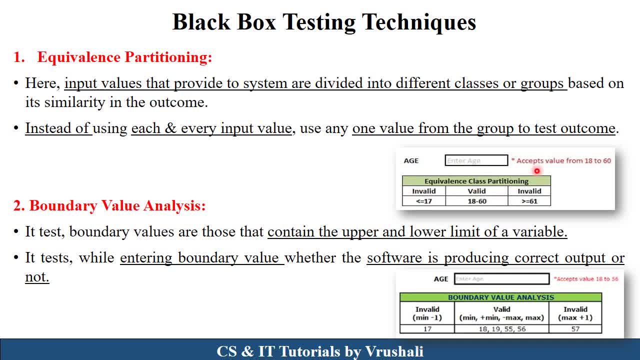 into the different group. For example, see here: Suppose they accept the value of 18 to 60 age Right Means. this is a valid group, This is a valid entry. Now, which are the invalid entry? Less than equal to 17 age, that is invalid. and greater than equal to 61 age. 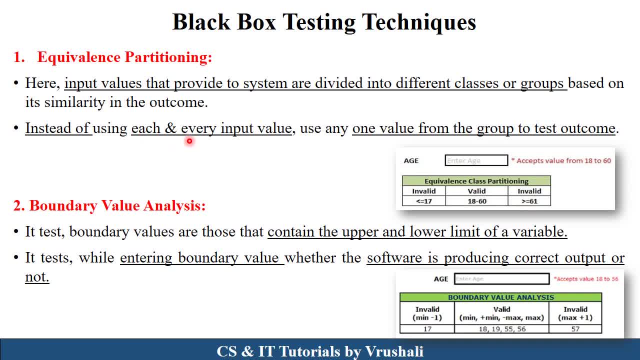 that is invalid Right. So instead of using each and every input value for testing purpose here, test one value from any group for testing purpose, That particular this age text box generate a proper outcome or not. This is called as equivalence partitioning technique. 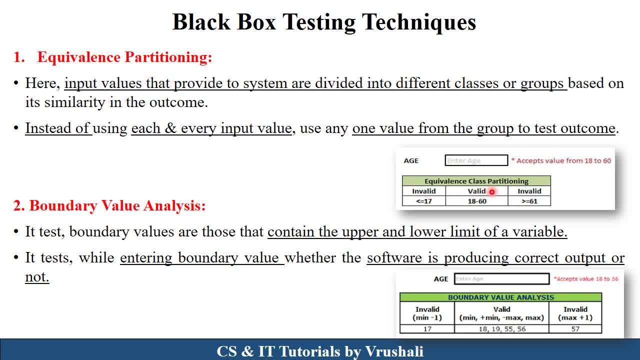 They partition your input value into different groups. The next technique is boundary value analysis. Boundary value analysis contain upper and lower limit of a variable or of the input value. See here in this example. The same example is there. Suppose in registration form there is a age option and this is a text box, So they accept the value only 18. 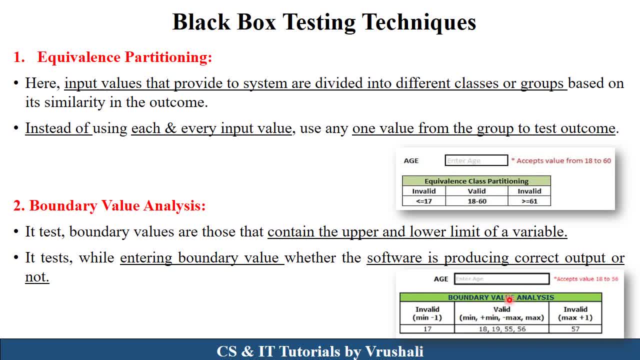 to 56 age only. Right Now in boundary value analysis there is a invalid, valid and again invalid. These three partitioning are there Now. valid means 18 to 56. This age is valid, which is acceptable by this text box Right Now. invalid means minimum minus 1. See here Minimum, 18 or maximum. 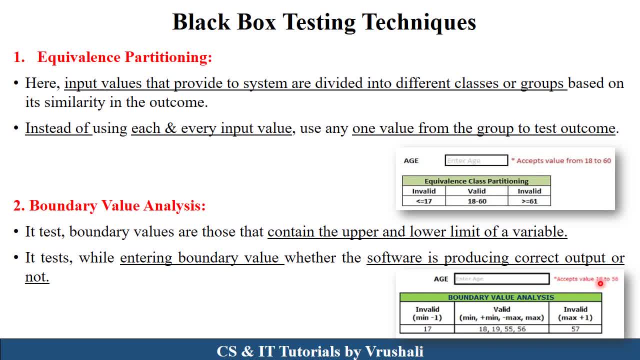 56.. So invalid means minimum minus 1. Means 18 minus 1,. 17 or below 17 are the invalid input. Now maximum minus 1. Means 56 plus 1. That is 57. So 57 and greater than 57, which is: 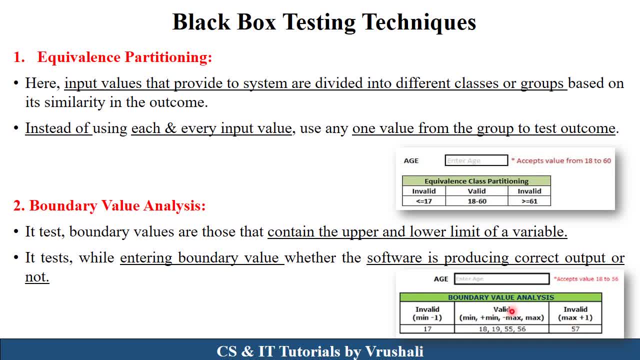 invalid input for this age Right Now valid. So again valid. there is a minimum plus minimum. Means: minimum value: 18 plus minimum means 19.. Maximum 56 and minimum maximum is 55.. Means: this is a boundary of each and every input value. So by entering this boundary, 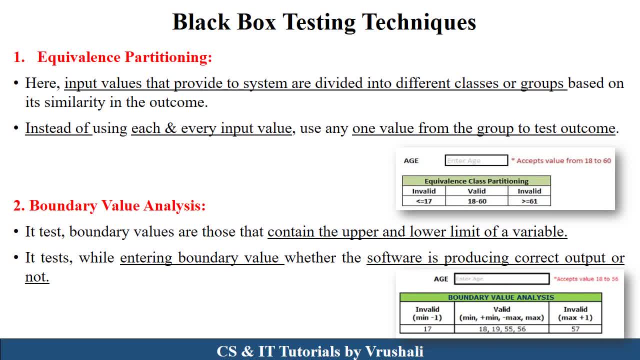 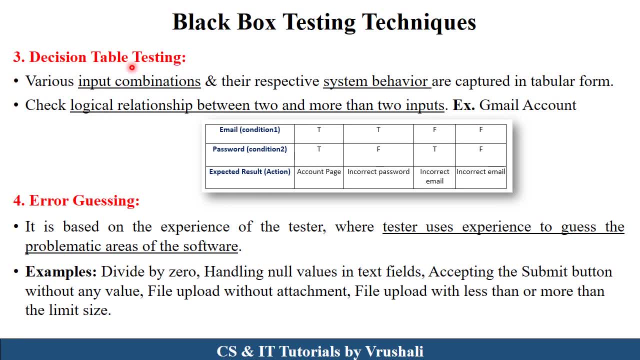 value tester. check that Your software is producing a correct output or not. Now the next technique is decision table testing. Let's take an example of your Gmail account. See, while logging a Gmail account, you can use a proper email ID and password. 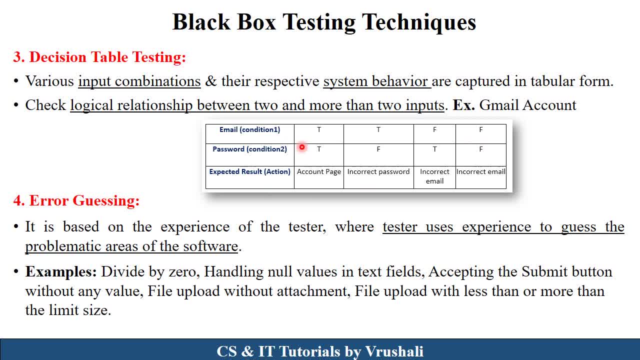 Right Now in this decision table. see here. Suppose you correctly enter email and password, Then your Gmail account page will be open Right. Suppose you entered email and password, Then your Gmail account page will be open Right. Suppose you entered email and password, Then your Gmail account page will be open Right. 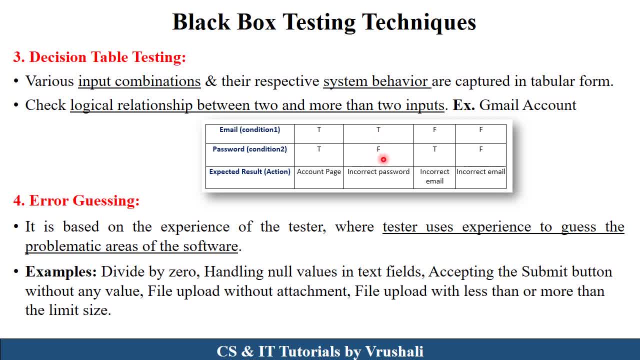 correct email id that is true or false and wrong password, so they will show the error incorrect password. suppose you enter wrong email id and correct password, so they will show you the error incorrect email. and suppose you enter wrong email id and wrong password, so they will give your error. 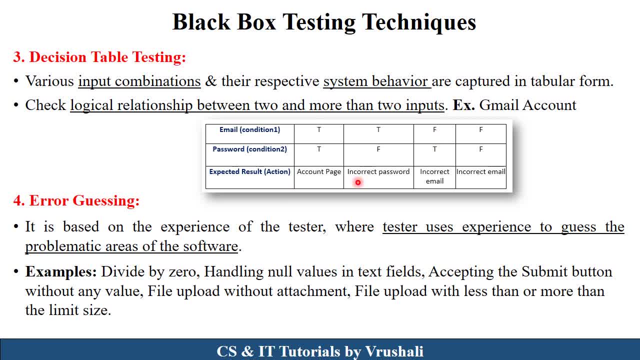 incorrect email. so this is called as decision table. here tester identify different input combinations and system behavior of the particular product. the next technique is error guessing. see tester having a different types of product testing experience, right. so for that purpose they use some guessing techniques for which type of errors will be generate in particular product or in particular. 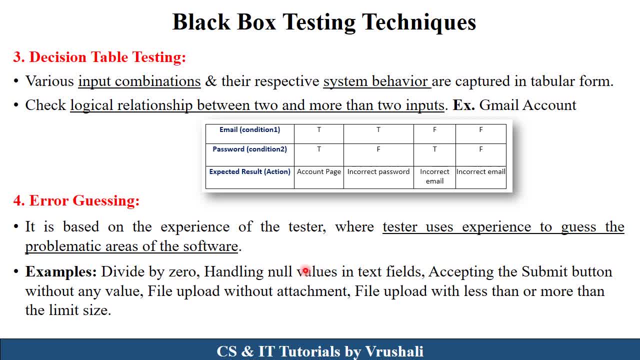 module like divide by zero error. is there then handling null value? for example, in suppose in registration system there is a mobile number error is compulsory to enter mobile number value, but still you submit a particular registration form without entering a mobile number, then they will show you the error right. then also file upload. 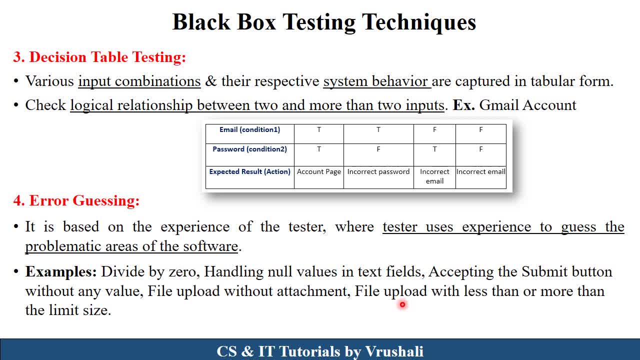 without attachment, then in particular registration form, passport size, photo size is confirmed, means only 10 kb size is required, right? so suppose you enter file upload with less than or more than limit size, then particular error will be generated. so this is called as decision table here. tester. 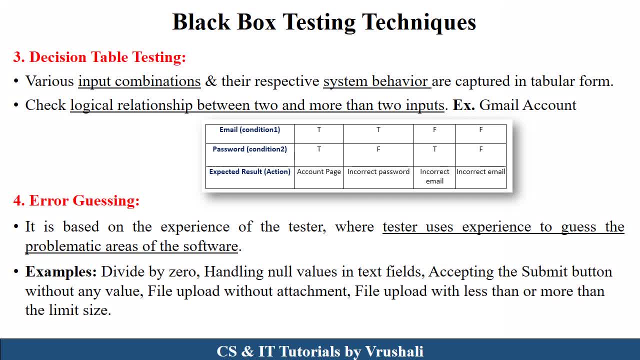 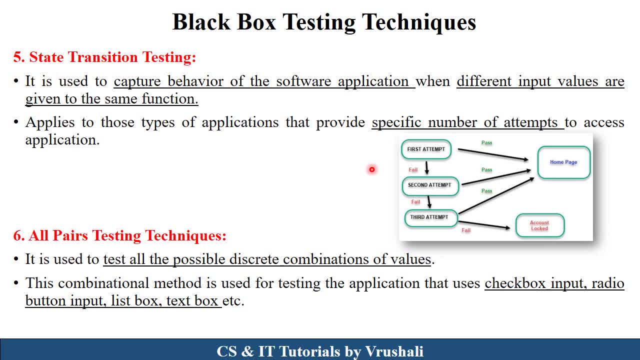 will be generate right. so this is called as error guessing. now the next technique is straight transition testing. see here: suppose why login a particular account. suppose when you login a Facebook account and you enter a three-time wrong password. so after entering fourth time, your particular account have lock right. so this is called as straight. 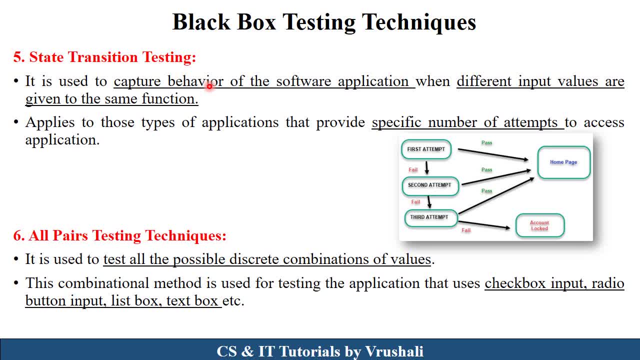 transition testing. in state transition testing tester capture a complete behavior of particular software product. they try different input values or, in particular, functionality, and only specific number of attempts are given. see here in this diagram: first attempt, second attempt and third attempt. you enter a wrong password and after that your account will be locked right. 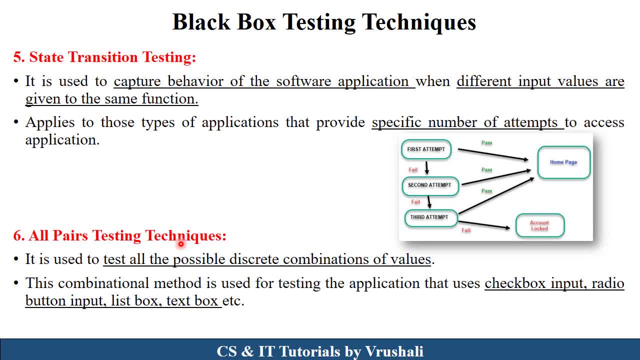 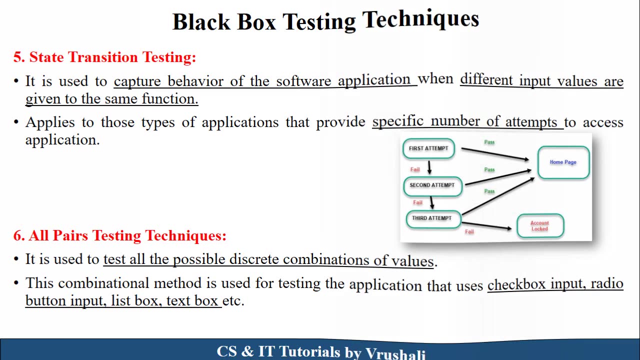 the next technique is all pair testing technique. basically here tester test all possible discrete combination values. suppose in registration form there are different check box, radio button, list box, text box. this kind of components are there for accepting the input values. so tester, they check that all these combinations are work properly or not. now the next topic is advantages of black. 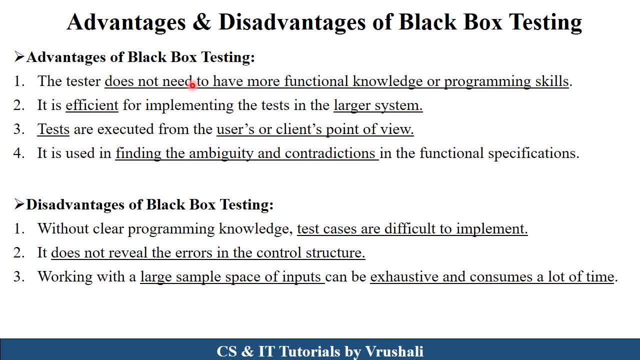 box testing. the main advantages is: tester does not need any functional knowledge or programming knowledge for testing purpose. and this black box testing is efficient when there is a large scale project is there and here tester generate a test cases as per the client requirement, whether a particular project generate a proper input and output as per the customer requirement or not. 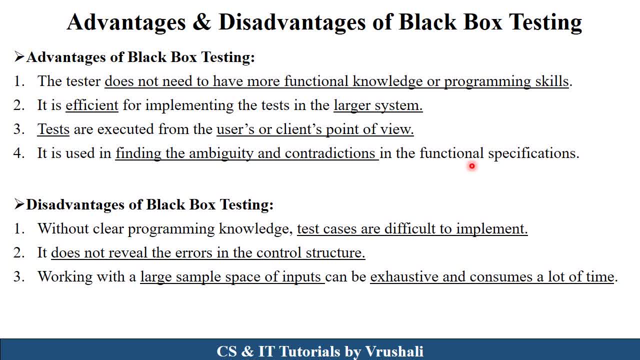 they also find out any contradiction in functional specifications. now, the disadvantages of black box testing is, without having any programming knowledge some time to generate a test cases or to write test cases. they will not be able to write test cases. they will not be able to write test cases. 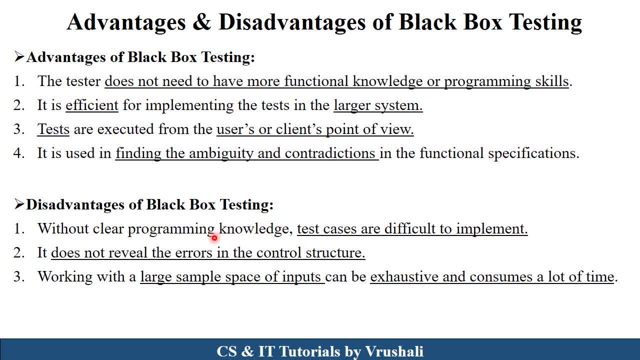 is very difficult, right. next thing is it does not reveal the errors in control structure or in programming language. they mostly focus only on input and expected output of your project. now, sometime, there is a large sample space of input or large group of input is there, so at that. 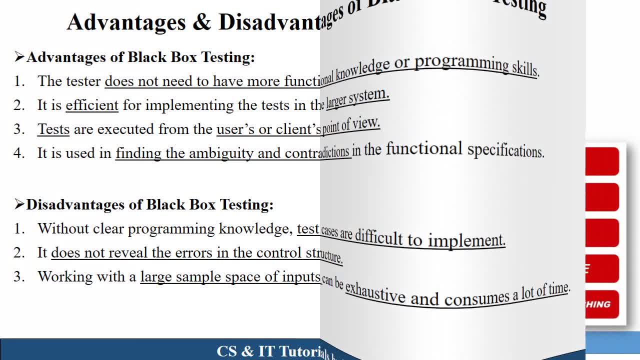 time. it consumed lot of time for testing purpose. so this is all about black box testing. thank you, keep learning you.